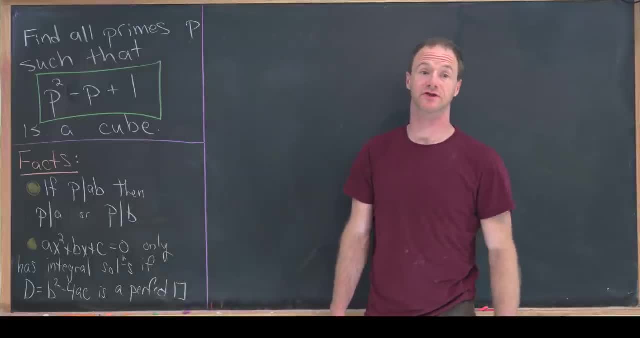 I've got a really nice number theory problem today, involving primes, to show everyone. So our goal is to find all primes, p, such that p squared minus p plus one is a perfect cube. We're going to use two fairly elementary facts along our journey. What's nice about these? 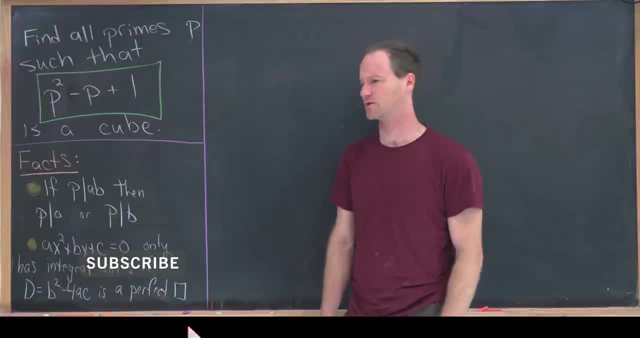 these are really elementary facts that you learn in like a high school algebra class or that are like kind of common knowledge and nothing involving like Fermat's Little Theorem or other tricks that happen in number theory type problems. Okay, so, first of all, if p divides a, b 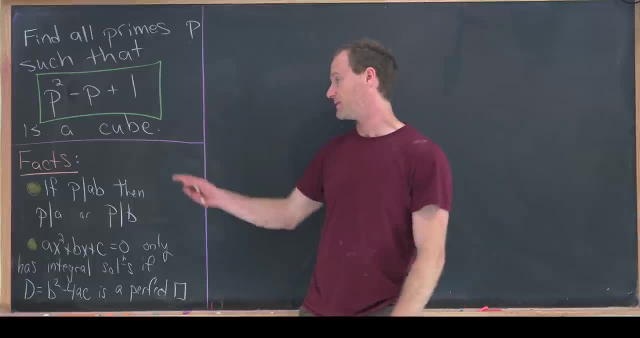 where that a, b is a product of the numbers a and b, then that means p divides a or p divides b, and that's of course assuming that p is a prime. And then the quadratic equation ax squared plus bx plus c equals zero, And then the quadratic equation ax squared plus bx plus c equals zero. 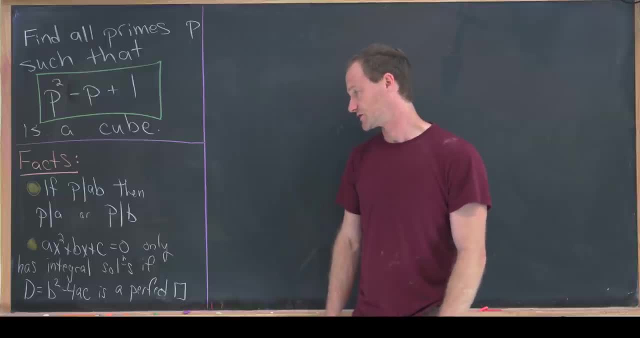 And then the quadratic equation ax squared plus bx plus c equals zero. And then the quadratic equation zero where a, b and c are integers, only has integral solutions if the discriminant, which is b squared minus 4ac, is a perfect square, So that discriminant is the thing that's under the square. 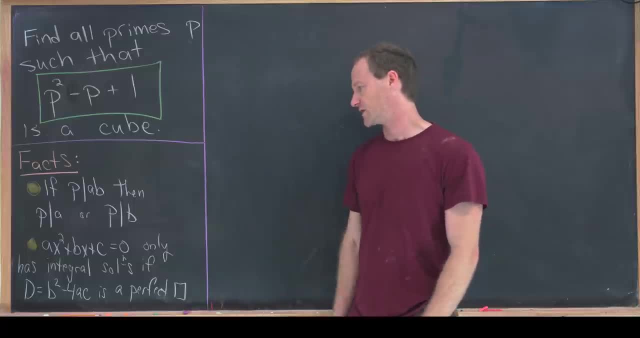 root in the quadratic formula. So I'll let you guys think about that. That doesn't tell you that the solutions are integral. They could still be rational, but we at least need that to be true to have integral solutions. So let's maybe get going, Let's take this stuff that's in the 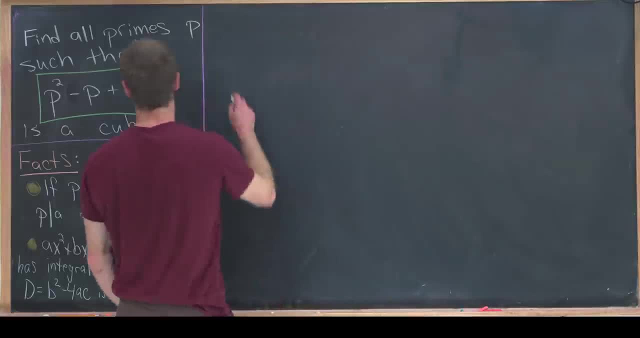 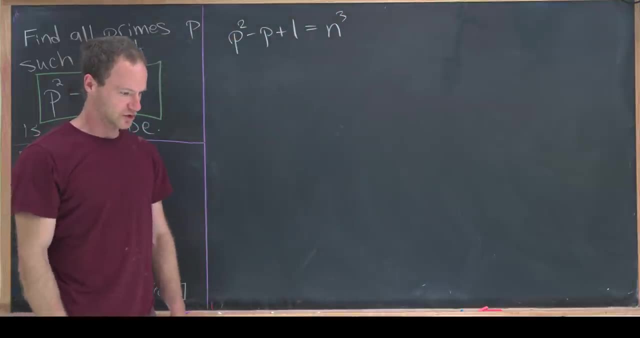 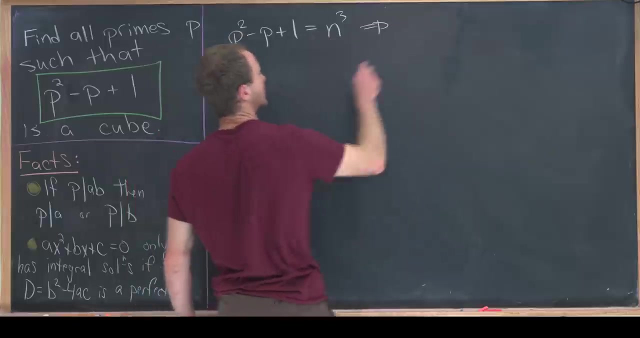 green box and set it equal to a perfect cube. So we've got p squared minus p. plus 1 equals n cubed. I would probably like to rearrange this so that we can easily factor these things. That's exactly what we'll do, So I'll subtract 1 from both sides of this equation. That gives me p squared minus p. 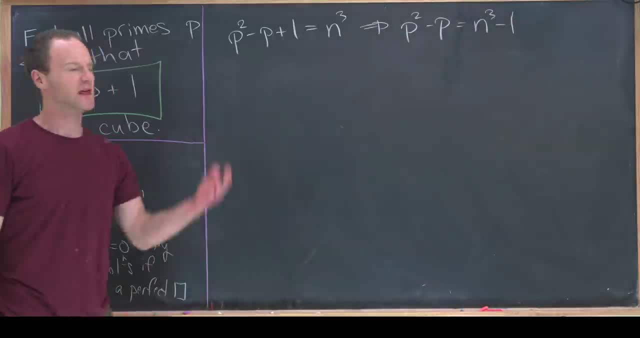 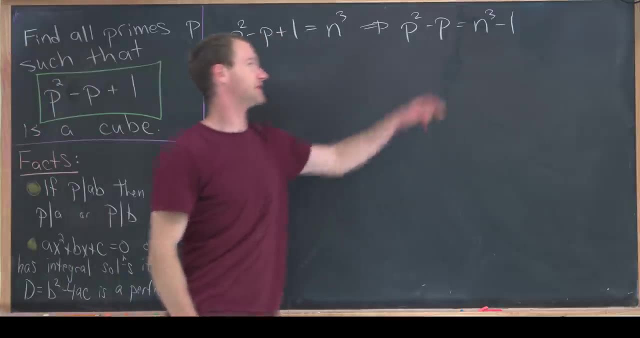 is equal to n cubed minus 1.. And then I've got a kind of straightforward way to factor both sides of this equation. So I'll subtract 1 from both sides of this equation. That gives me p squared. this is like a difference of cubes. and then we've got a greatest common factor of p over on the left. 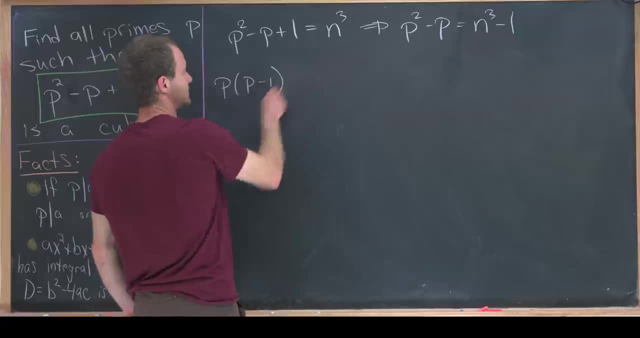 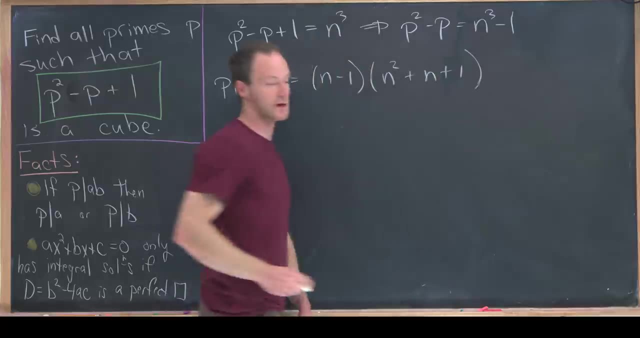 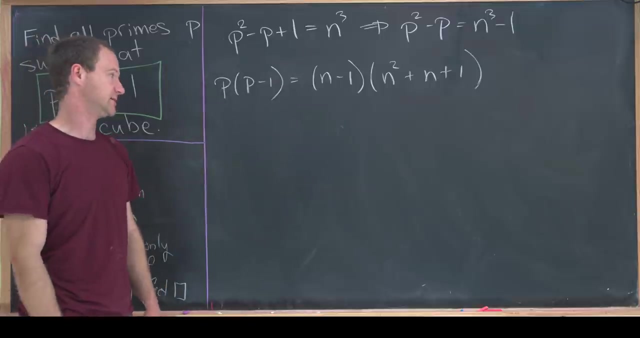 hand side. So now we have: p times p minus 1 equals n minus 1 times n squared plus n plus 1.. But now notice: p divides the left hand side. That means p divides the right hand side. But if we think about this playing the role of a and this playing the role of b, that means p must divide either a. 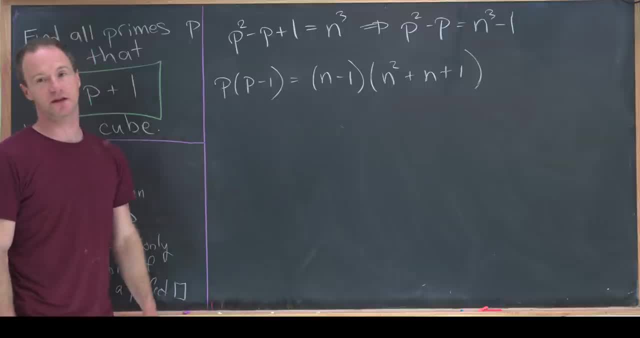 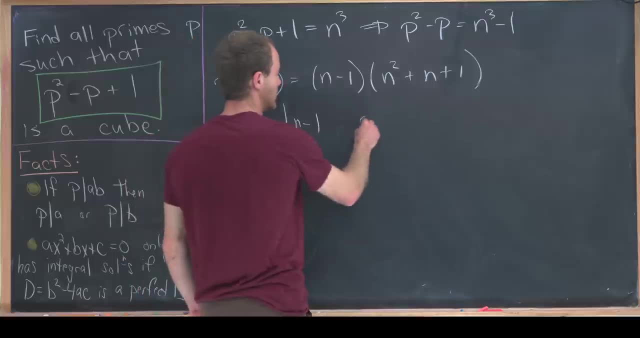 or b, In other words either n minus 1 or n squared plus n plus 1.. So let's maybe note that. So note that p divides n minus 1, or p divides n squared plus n plus 1.. Now let's actually show. 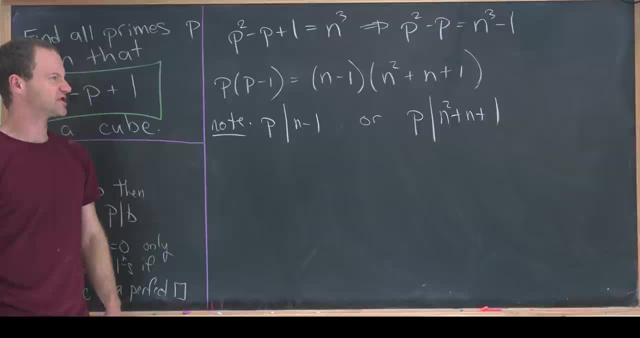 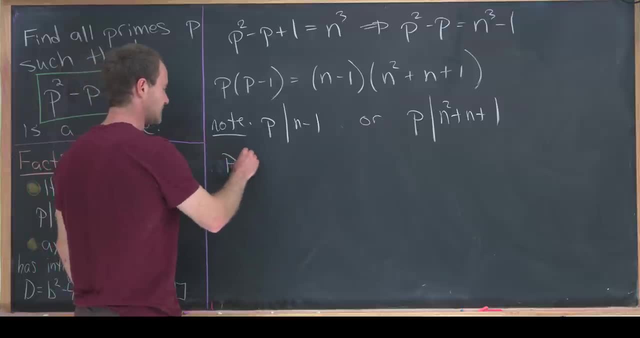 that this is impossible, and we can do that just by playing a game with inequalities. So let's first notice that if p divides n minus 1, that means p is less than or equal to n minus 1.. So let's hang on to that and then notice that p cubed is most definitely bigger than p squared. 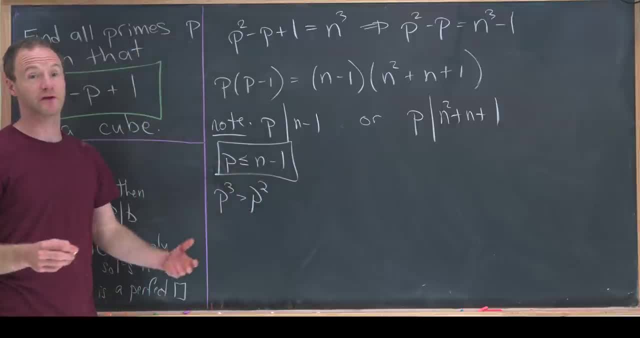 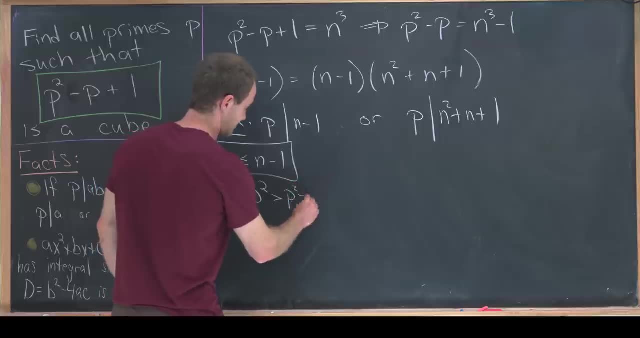 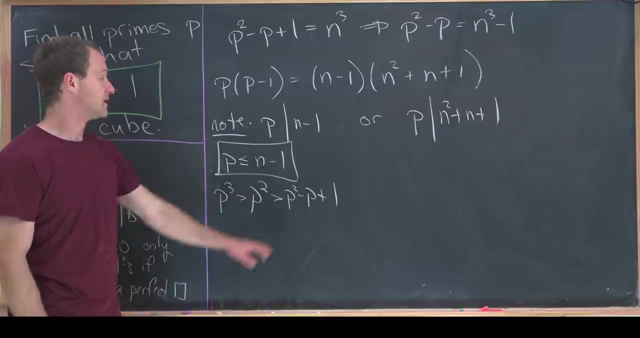 That's because p is a prime, making it bigger than or equal to 2.. But now p squared is bigger than p squared minus p plus 1.. That's because minus p plus 1 is going to be less than 0.. Again, because we have a prime there. But now that's equal to n cubed. But now, looking at the, 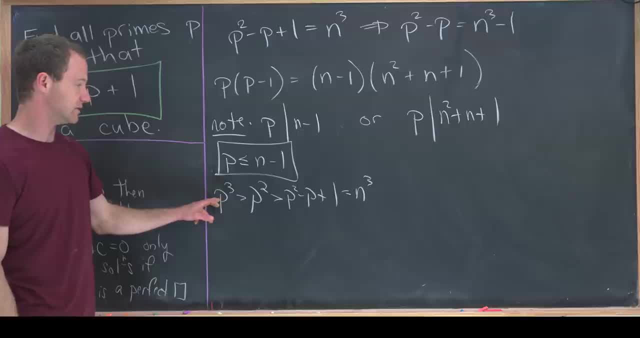 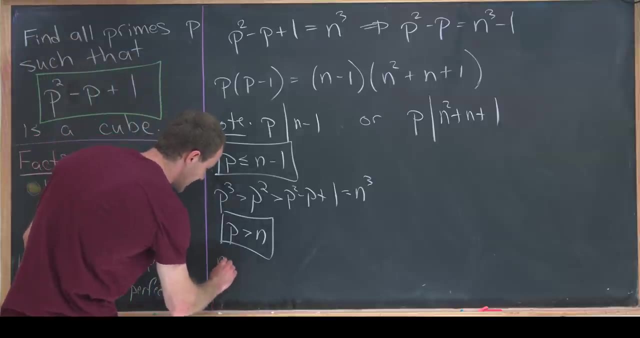 extreme left and right hand side of this equation, we see that p cubed is bigger than n cubed, which means that p is bigger than n, But now we can put these two boxes together into a bit of a contradiction. So let's notice now we have: n is less than p, which is less than or equal to n minus. 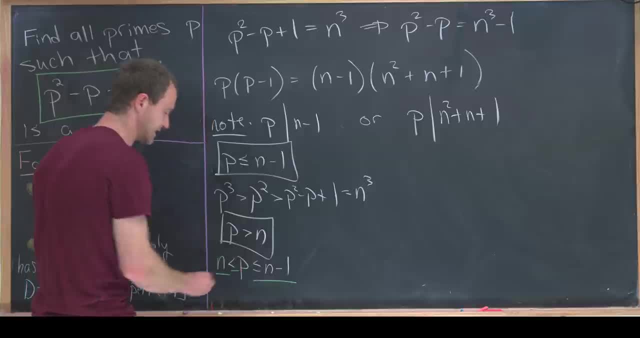 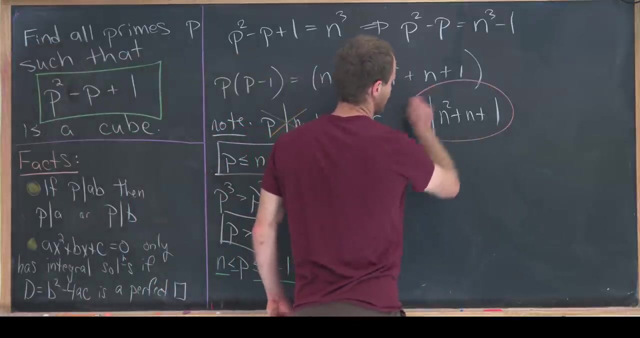 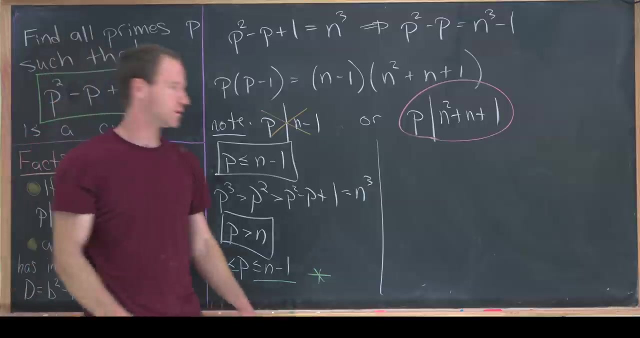 1. Which tells us that n is strictly less than n minus 1, which is a clear contradiction. So that means it is impossible for p to divide n minus 1.. But that means that this possibility over here is really our only case that will work. We have: p divides n squared plus n plus 1.. 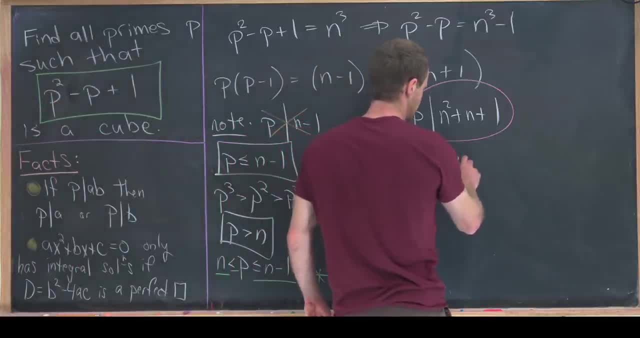 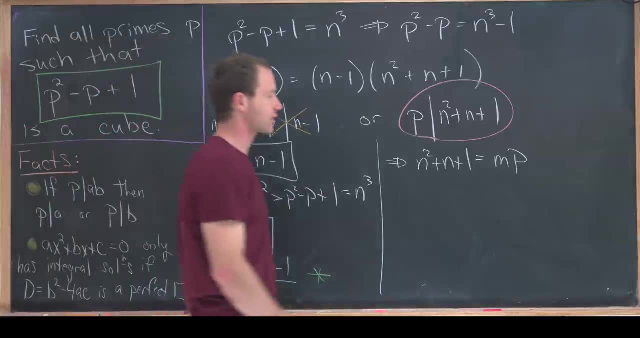 In other words, we can write n squared plus n plus 1 as a multiple of p. We'll call it m times p for obvious reasons, And now we're going to throw this into. This is not only our original equation, but one of our first equations. 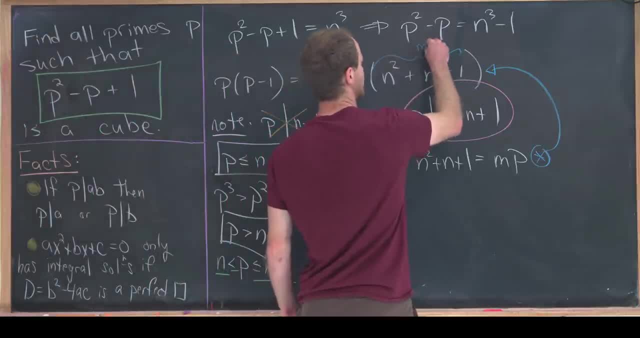 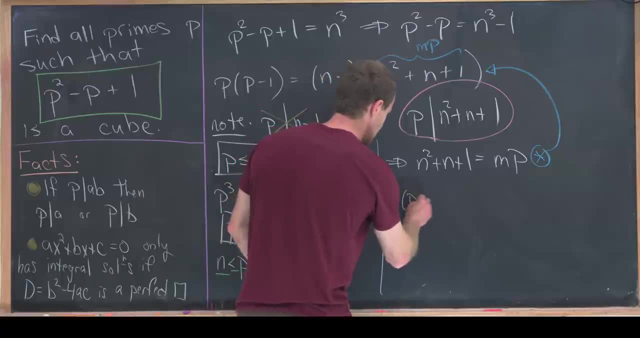 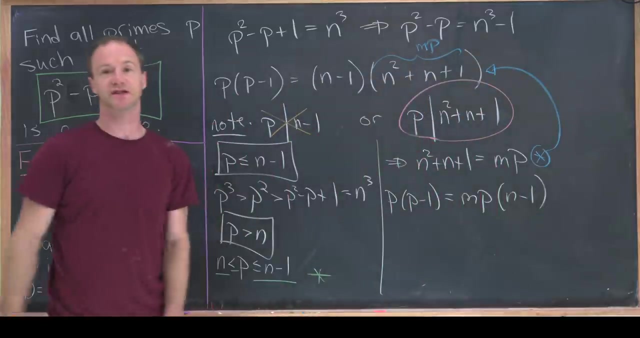 Noticing that we can take all of this and replace it with m times p, which maybe makes the whole thing look a little simpler. Let's see what we've got now. We have p times p minus 1 equals m times p times n minus 1.. I've just rearranged things a little bit, But we can cancel p from both sides. 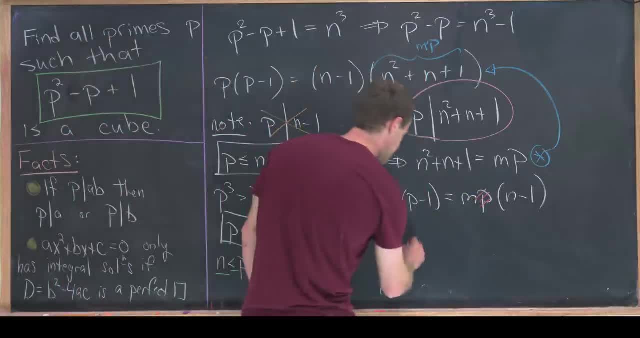 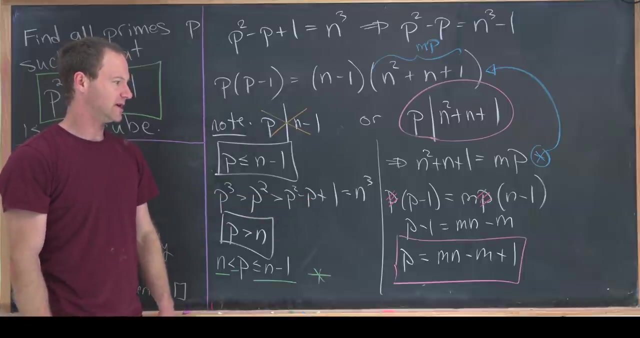 of this equation just by dividing by p, And that tells us that p minus 1 is equal to mn minus m. Alright, But that means that p is equal to mn minus m plus 1.. So now we've got this expression for p in terms of m and n. Now we'd like to take this expression and maybe plug it back. 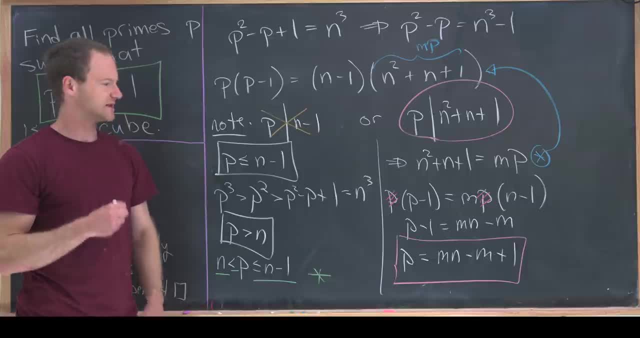 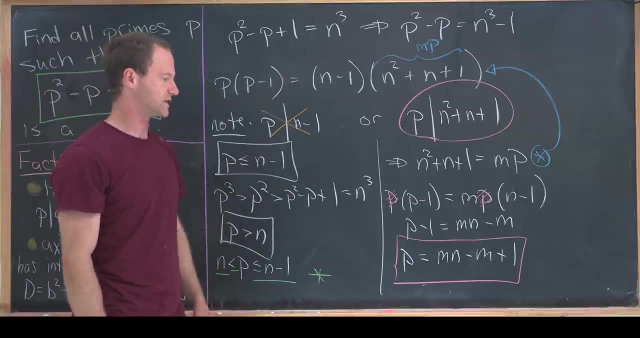 into one of our earlier spots and see if we can maybe use that to solve for m or n. And that's exactly what we'll do. But we'll do it on the next board Because we're running out of room. we'll take this value of p and throw it back up here and see what. 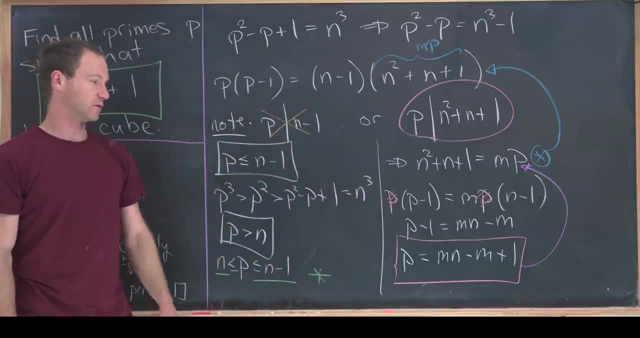 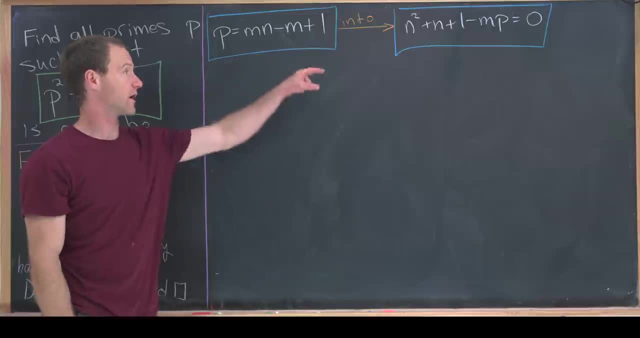 we get. Okay. So let's maybe get rid of this and we'll make that substitution. So on the last board we determined p in terms of n and n, where those also satisfy this equation. right here We've got n squared plus n, plus 1, minus mp equals zero. Now we're going to plug this value of p into. 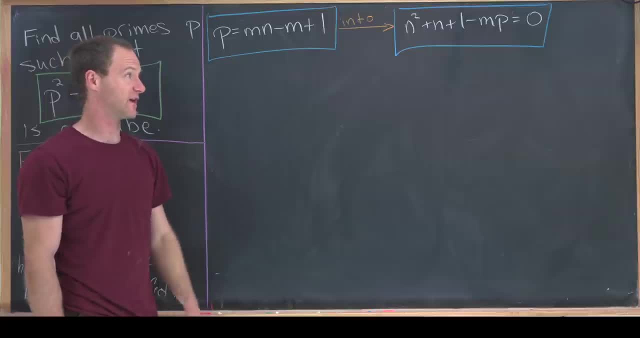 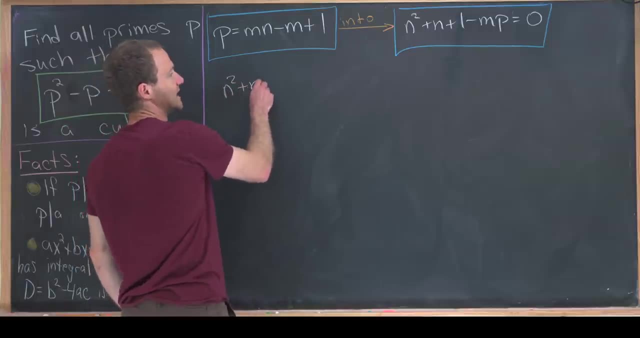 that equation over there Which, remember that, came from the first equation we solved for p. So remember that came from the fact that p divided that n squared plus n plus one object. So let's see what we get. We'll get n squared plus n plus one minus m times p. So that's going to be minus m squared n plus m. 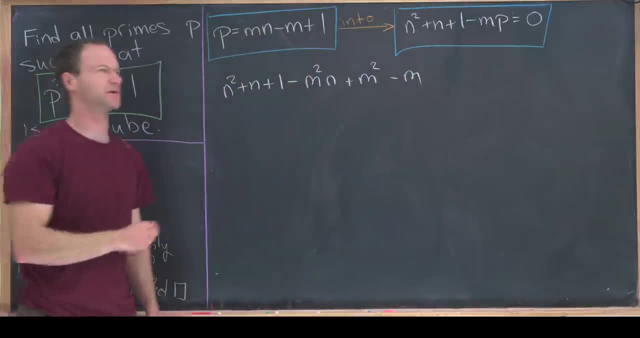 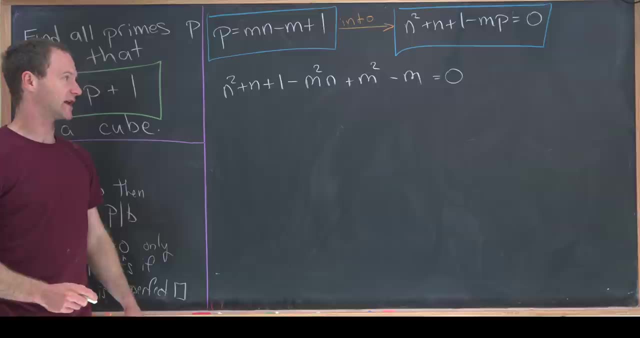 squared minus m. So I get that just from distributing a bunch of stuff. So we've got: this is equal to zero. But now notice that this is quadratic in m and n. So it stands to reason that we could use the quadratic formula, viewing m as a variable and n as a constant, or vice versa. 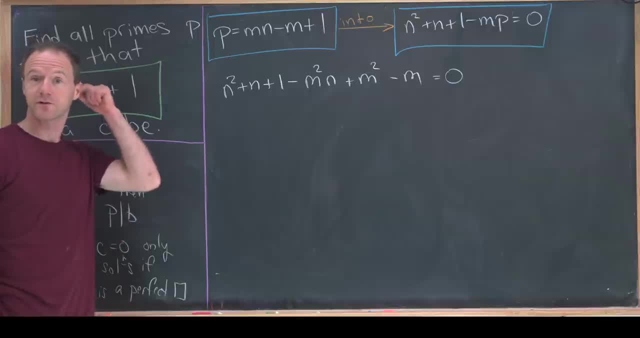 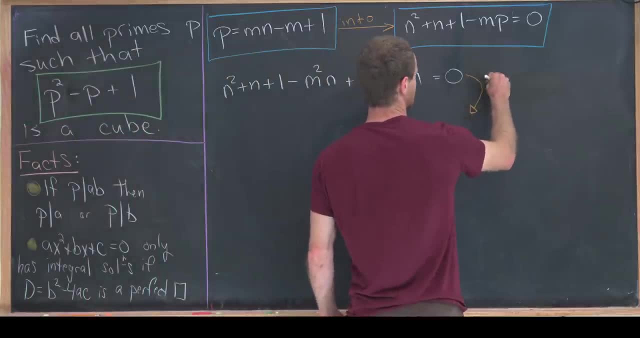 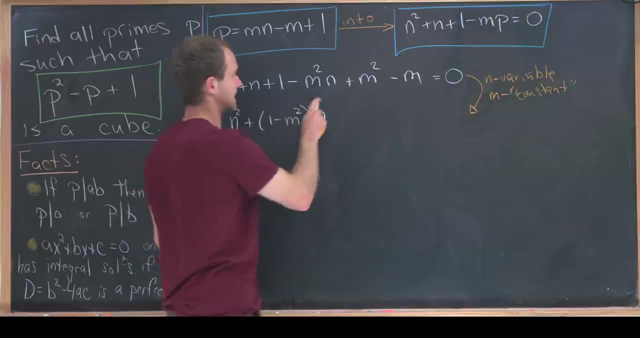 to get an idea for what are the possible values for m and n. That's exactly what we'll do, So we'll start off by viewing n as a variable and m as a constant, And that allows us to rewrite this as n squared plus one, minus m, squared times n, and then plus m squared minus m. 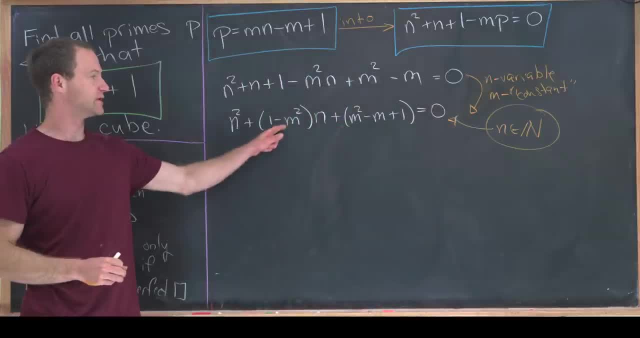 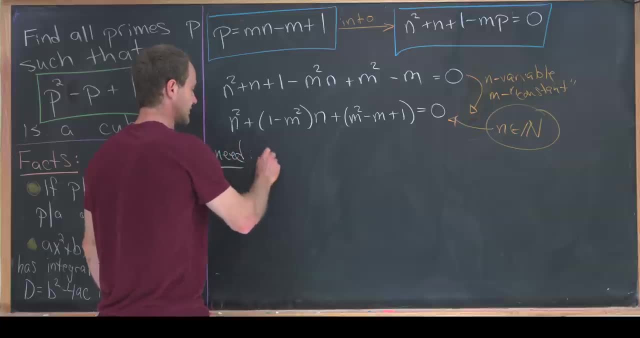 plus m squared times n. So we'll start off by viewing n as a variable and m as a constant. plus one equals zero, like that. But that means we need the discriminant of this object to be equal to a perfect square. So let's write that down. So we need the discriminant. I'll call that capital. 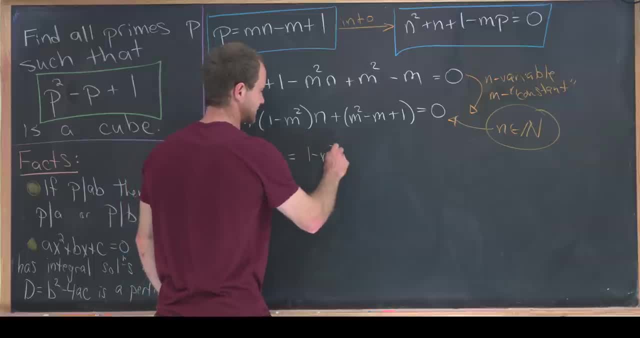 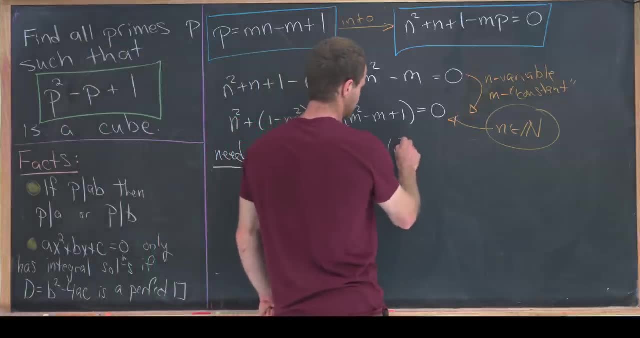 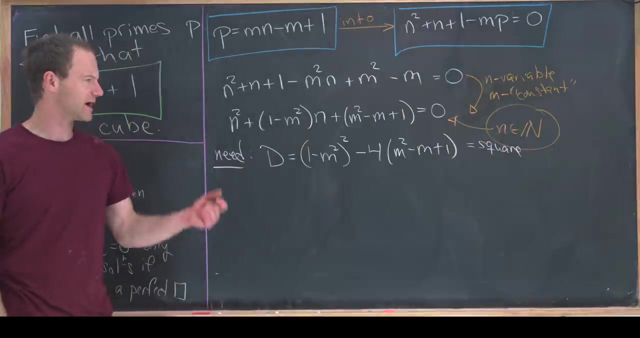 d, which is this: b squared one minus m squared, squared minus four times a times c. So that's going to be four times m squared minus m plus one, to be equal to a perfect square. Okay, well, that might look a little bit weird, But it's not. So let's start off by viewing n as a constant. 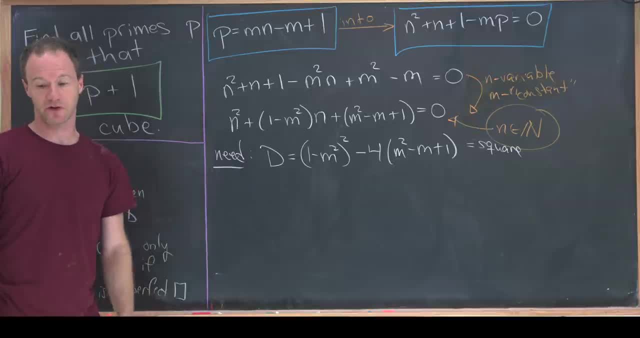 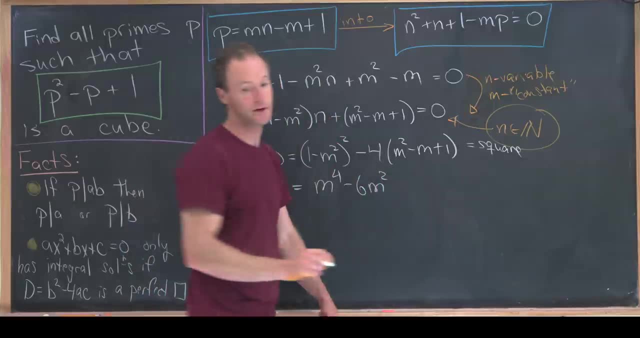 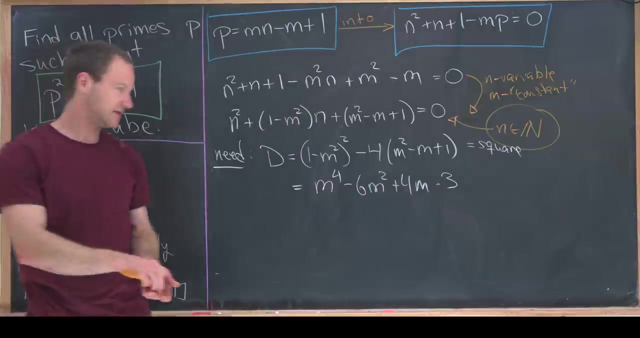 It's a little bit tricky to work with, But maybe we can expand it out and play some games. So notice that this expands out to m, to the fourth minus six m squared, and then plus four m minus three. Like I said, we need this object to be equal to a perfect square. 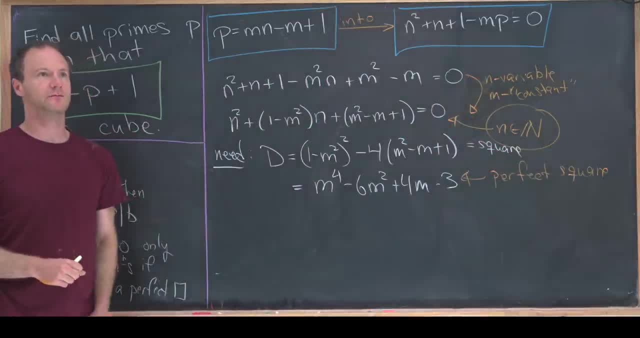 And what we'll do is we'll bound it between two consecutive perfect squares For all but finitely many values of m. And which two perfect squares should we play around with? Well, maybe we'll look at the first perfect square that will replicate. 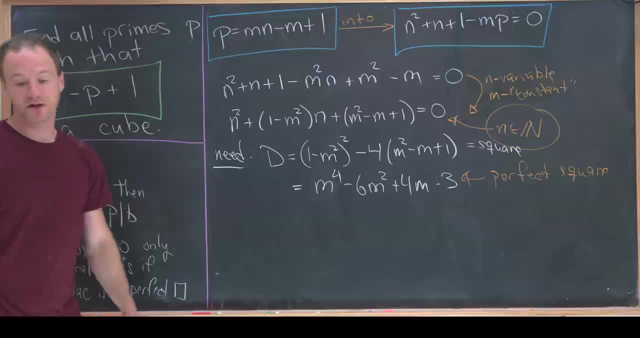 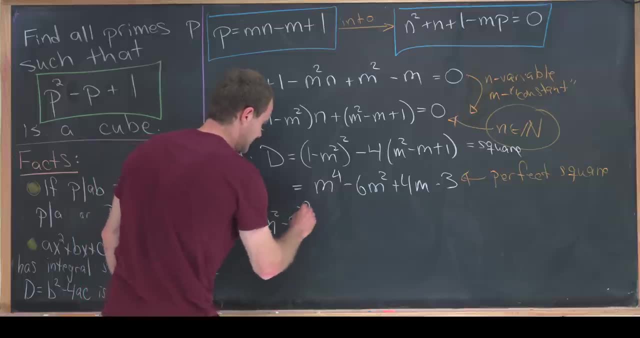 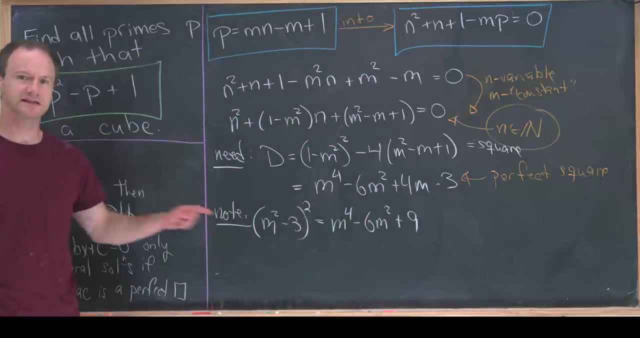 this first term and this second term. So let's do that. Maybe I'll write this as notice: if we take m squared minus three, quantity squared, we get m to the fourth minus six, m squared plus nine. Like I said, we wanted to replicate this first. 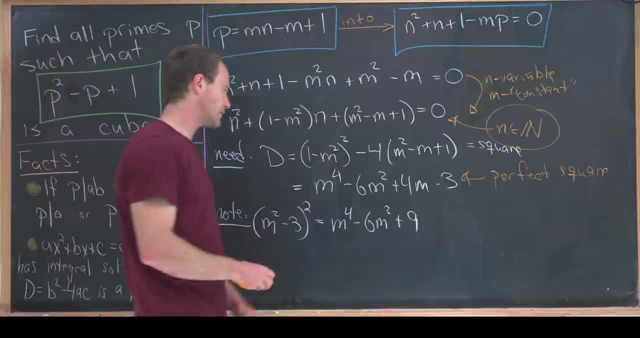 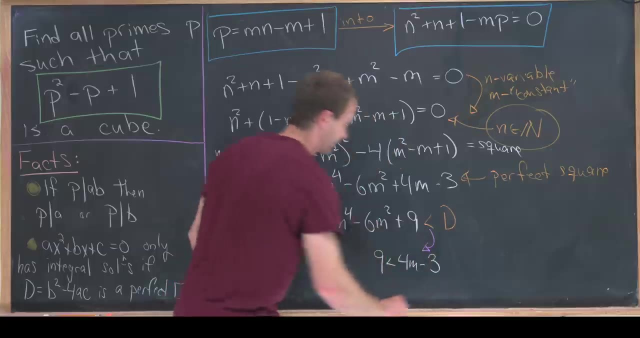 second term, and that's exactly what we've done. But what we want is for this to be less than our object, which is called d. But when will that happen? So that's going to happen when 9 is less than 4m minus 3, because we need this 9 to be less than whatever's left over over there. But that 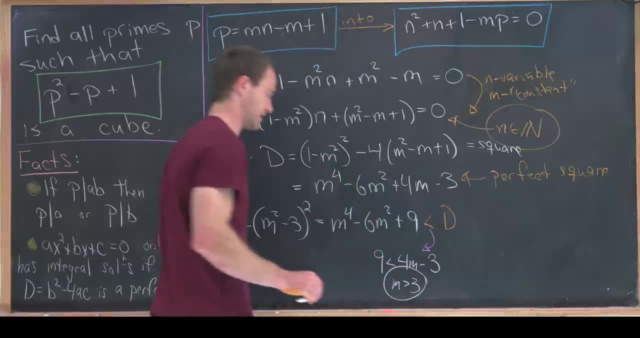 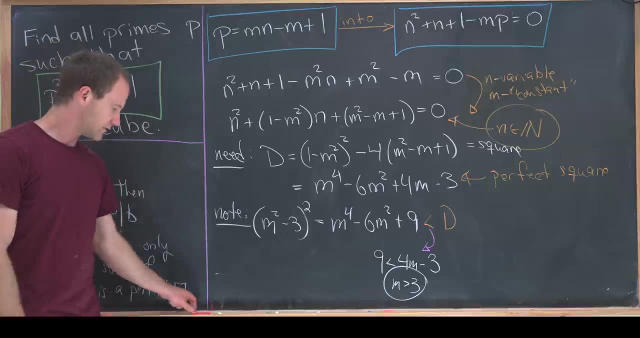 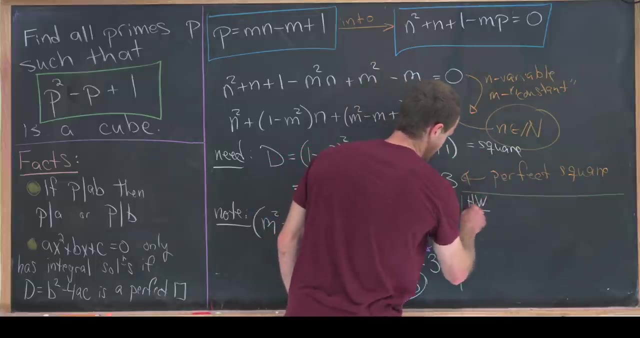 occurs when m is bigger than 3.. So we've seen that if m is bigger than 3, our discriminant is bigger than this perfect square. So that's not super helpful on its own, but combined with the other observation which I'll leave as a homework, which is actually a little bit simpler than this. 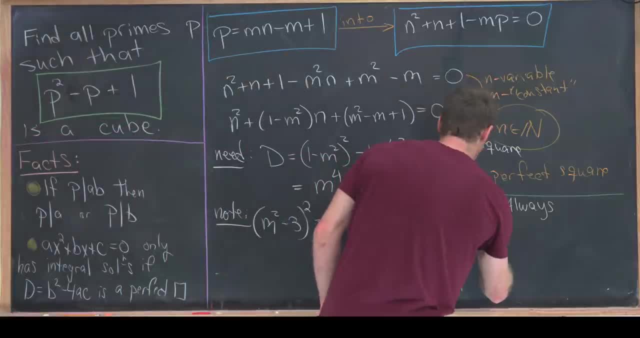 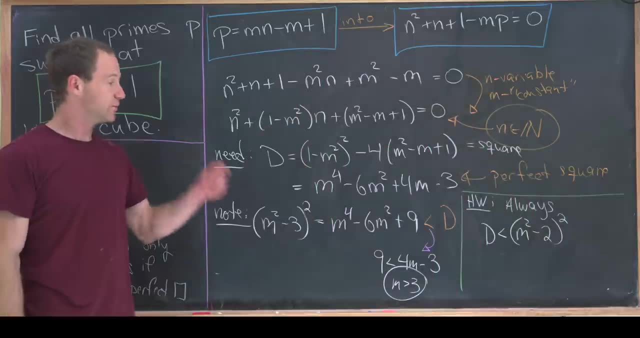 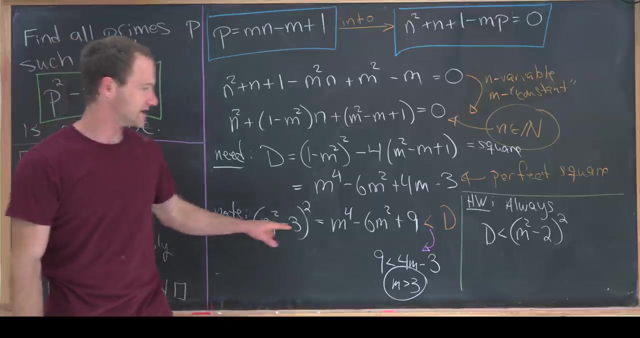 we'll see that always our discriminant is smaller than m squared minus 2 quantity squared. So putting that together we see that for m bigger than 3, the discriminant is perfectly between these consecutive perfect squares. But if it's perfectly between those consecutive perfect. 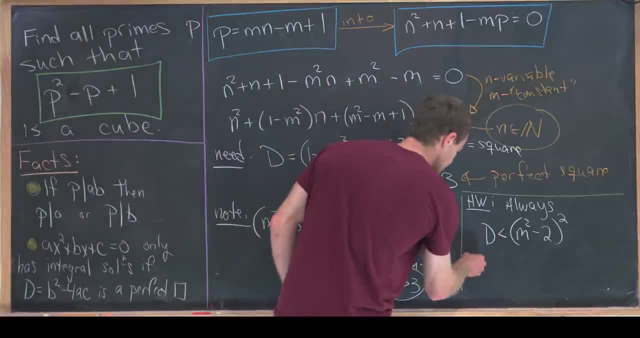 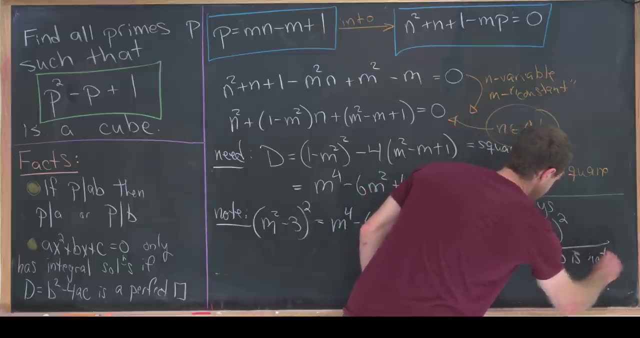 squares. that means it cannot be a perfect square. So let's write that down. So if m is bigger than 3, d is not a square. So that tells us that m must come from a square. So that tells us that m must come from a square. So that tells us that. 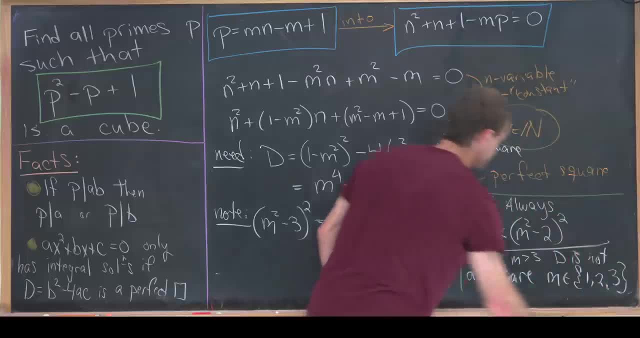 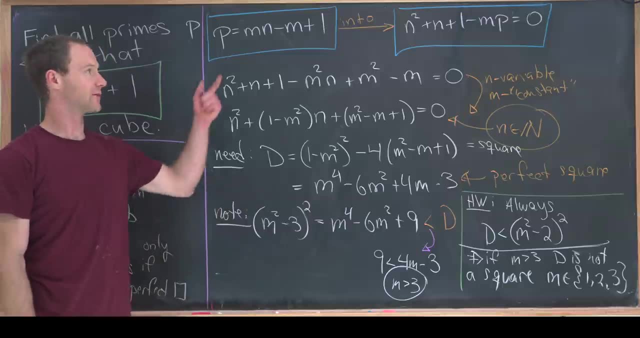 m must come from the set 1,, 2, or 3.. So notice, we have a strict inequality there. So it is possible for this thing to be equal to 3.. Okay, so let's summarize that at the top, and then we'll work. 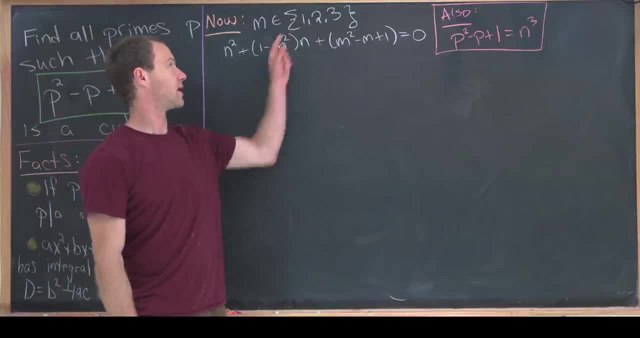 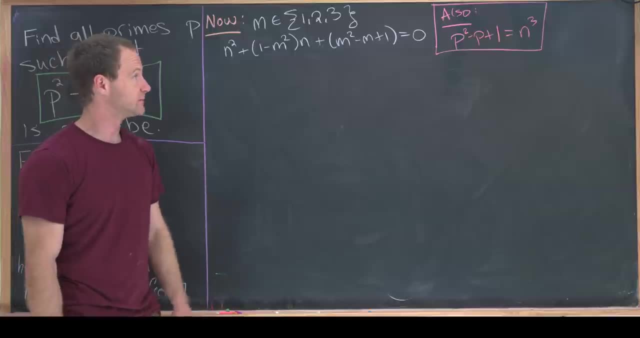 towards the end. So far we've determined. our possible values of m are 1,, 2, and 3.. Furthermore, n and m are connected by this quadratic equation, and then n and p are connected by that equation over there. So now we want to determine the difference between m and 3.. So we're going to 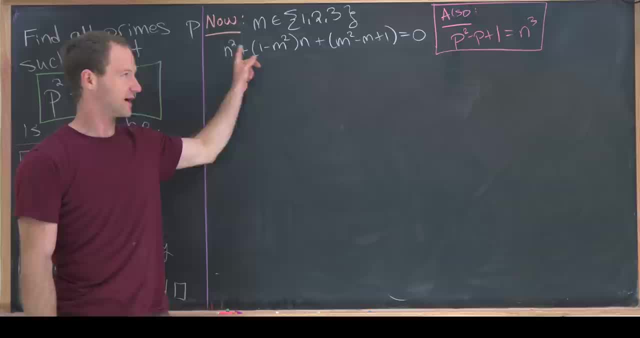 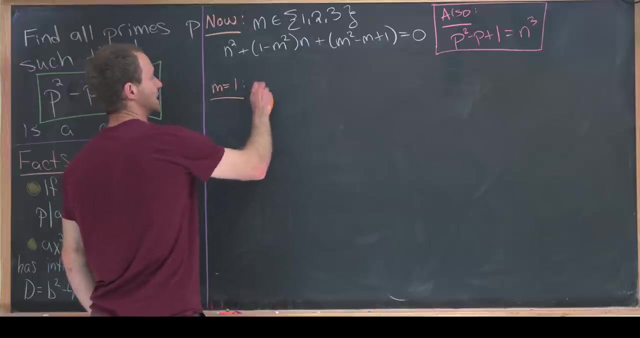 take the possible values of n and plug them over here and find the possible values of p, which is our final goal. Okay, so let's do this in a step-by-step process. So let's take m equals 1 first. So that means we're going to get n squared plus well, that turns into 0, and then plus 1 equals. 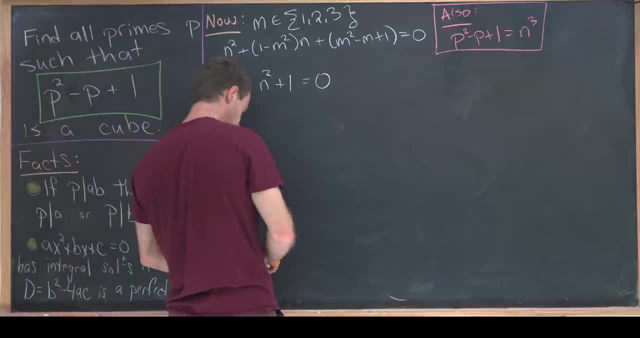 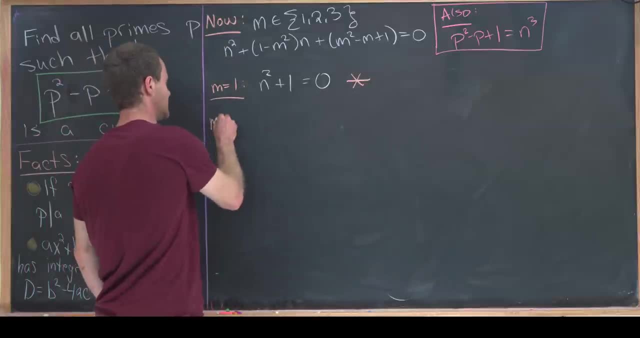 0. But notice: that has no integer solution. So we can just maybe put an x next to it, So we can. this has no solution. So now let's look at the case when m is equal to 2.. So here we're going to. 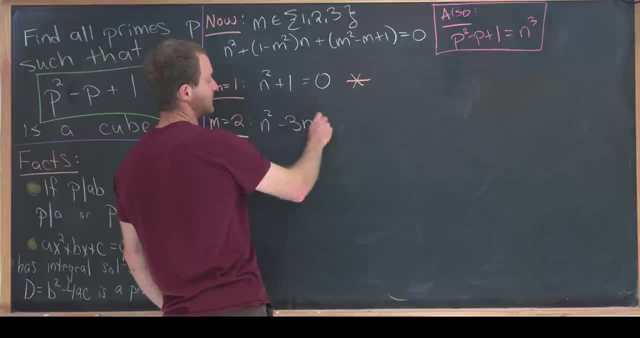 get n squared minus 3n and then plus, let's see what we have. We've got 4 minus 2 plus 1.. So that's going to be plus 3 equals 0.. Well, I'll let you guys check this as well. but this also has no.